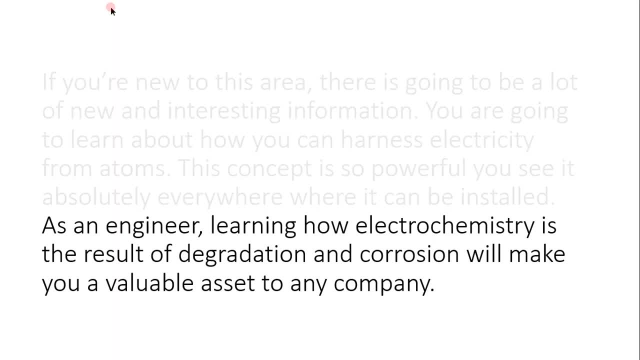 make you a valuable asset. I could have worded that better, but essentially what I'm saying is the result of degradation and corrosion in metals is a result of electrochemistry, but first you need to understand degradation and corrosion and dissolution and deterioration. Yeah, there's, there's a few ways that materials can not be that the material they were originally. 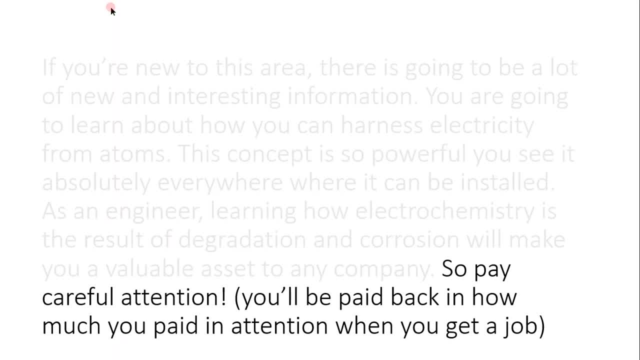 before. So pay careful attention and don't worry, you'll be paid back in how much you paid in attention when you get a job. So if you pay a hundred percent attention, guess what that's gonna reflect in your salary. That's my theory anyway. So everything in this universe is made. 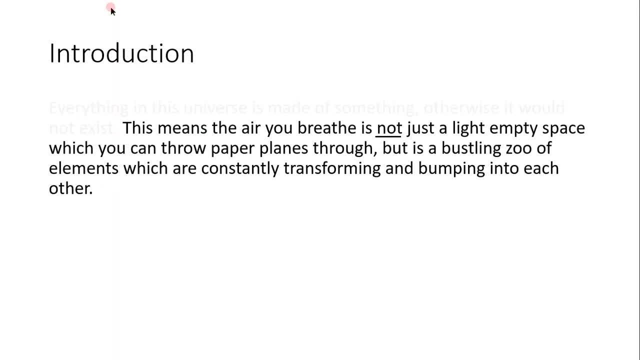 up of something, otherwise it would not exist. This means the air you breathe is not just a light empty space where you can throw paper planes through, but is a bustling zoo of elements which are constantly transforming and bumping into each other. This may not seem so fantastic. 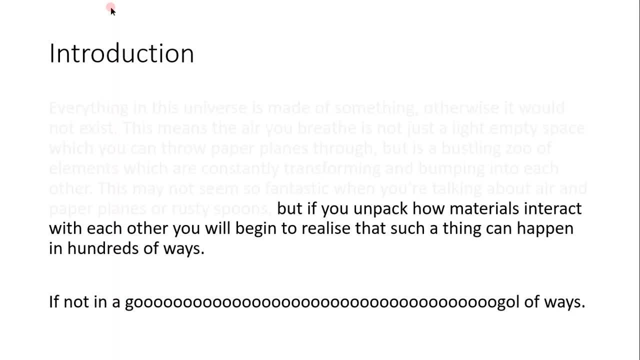 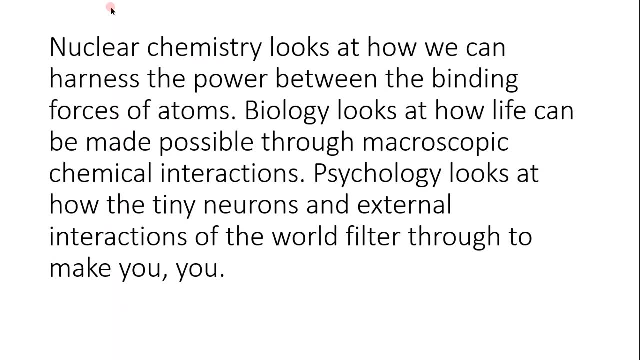 when you're talking about air and paper planes or rusty spoons. but if you unpack how materials interact with each other, you'll begin to realize that such a thing can happen in hundreds of ways, if not in a google of ways. So nuclear chemistry looks at how we can harness the power between 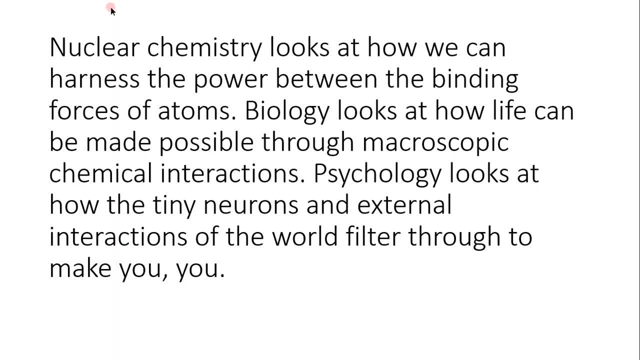 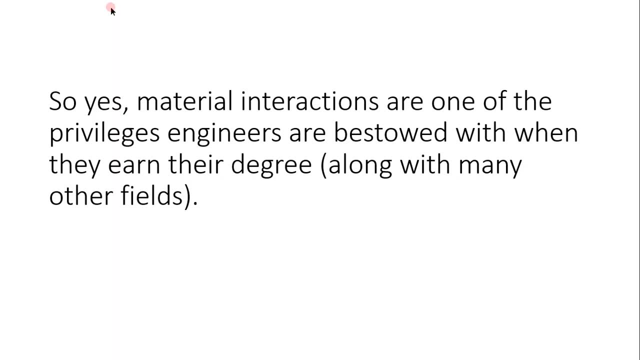 the binding forces of atoms. Biology looks at how life can be made possible through macroscopic chemical interactions, and psychology looks at how the tiny neurons and external interactions of the world filter through to make you you. So, yes, material interactions, one of the privileges engineers are bestowed with when they earn their degree, along with many 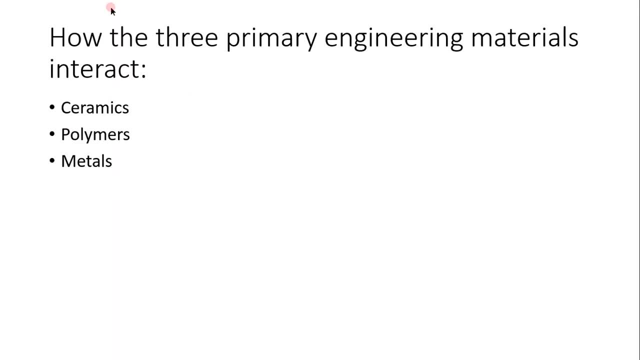 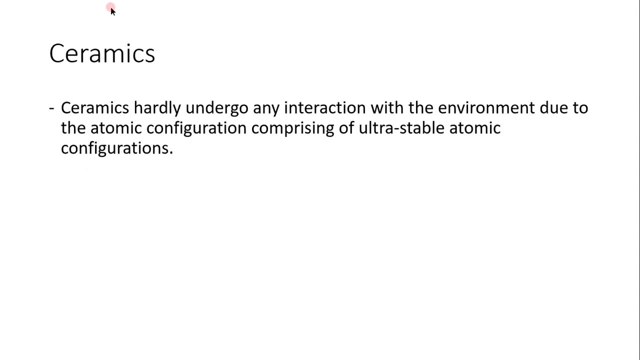 other fields. So we're going to look at how the three primary engineering materials interact, namely our ceramics, polymers and metals. Ceramics hardly undergo any interaction in the environment due to the atomic configuration comprising of ultra stable atomic configurations. They've got. 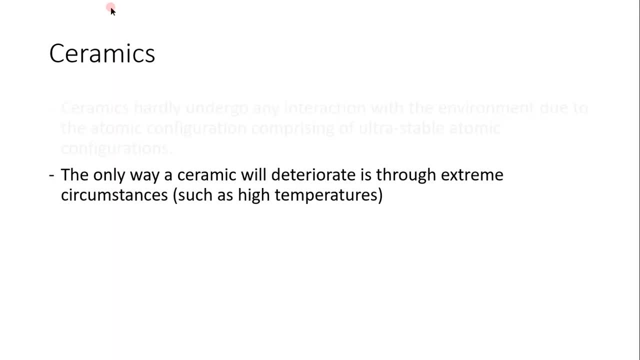 the most stable atomic configuration, so they don't really do much. but the only way a ceramic will deteriorate is through extreme circumstances. Polymers: they degrade, they don't corrode or deteriorate. this is important. So they often dissolve in solvents, they absorb solvents and they swell. 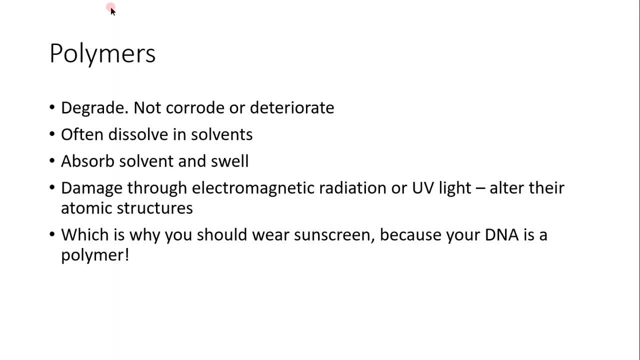 Sometimes they are damaged through electromagnetic radiation, or UV light, which is EMR, and this alters their atomic structures because they're relatively weak in comparison to ceramics, which is why you should wear sunscreen. because your DNA is a polymer. It will degrade. they don't corrode or deteriorate. this is important. 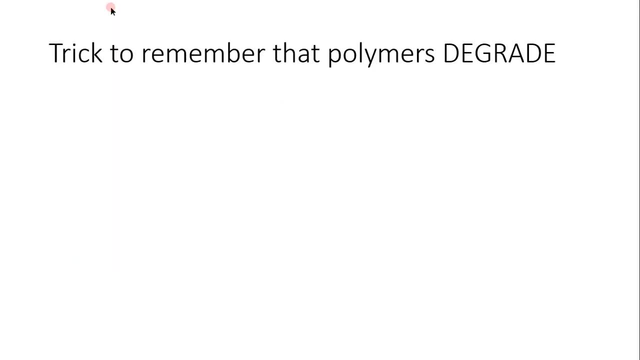 Polymers will degrade. if you don't cover up, you don't degrade. so this is a trick that i use to remember that polymers degrade. they don't deteriorate, they don't corrode, whatever. whatever. if you're an A plus student, your grades are said to be high. 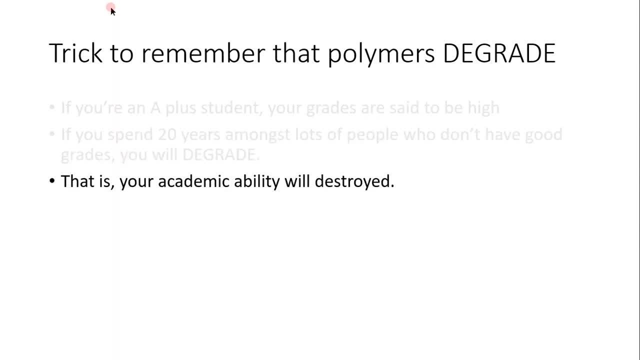 but if you spend 20 years amongst sorts of people who don't have good grades, you will degrade, that is, your academic ability will be destroyed. that's a bit. it's a bit of an exaggeration, but you know what i mean. just like the polymer, if you put it in an environment where it is surrounded by lots of degrading chemicals, it will degrade. 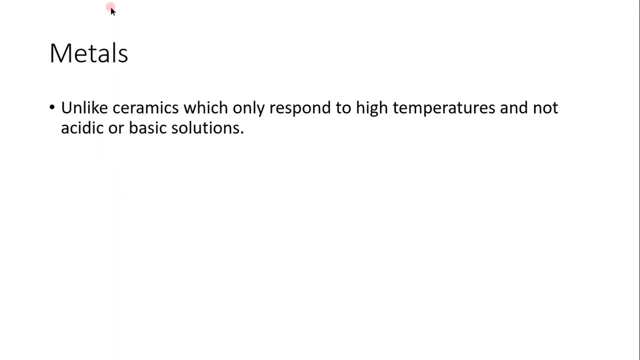 so if you put it in a room far behind a classroom or in a small hall, it will degrade. So onto metals Now. unlike ceramics, which only respond to high temperatures, are not acidic or basic solutions, because acids and bases donate protons as well as some electrons. 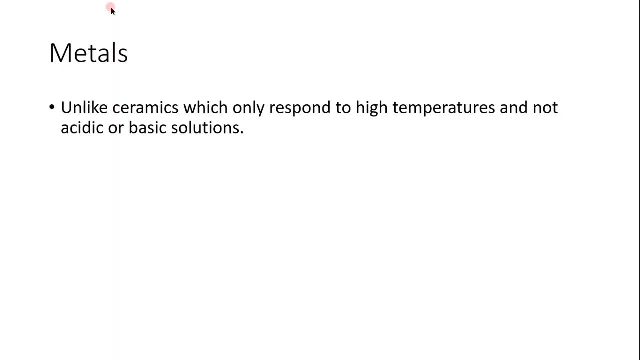 in some cases Ceramics, because their atomic configuration is so stable. just they don't do anything. And polymers: they do degrade due to alterations in their atomic structure because they're not as stable as our ceramics. They have room to accept protons against their 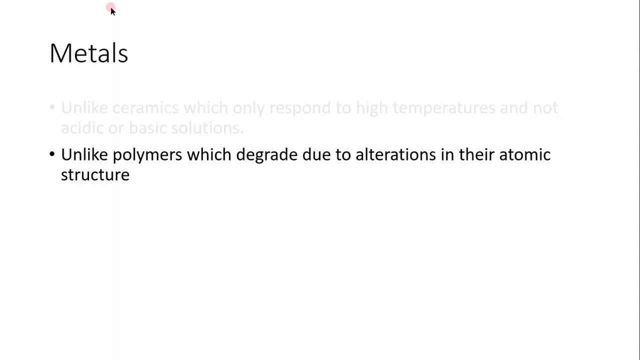 will. and yes, if they are hit with electromagnetic radiation, it will cause some bad things in the electron field. So that's right, wear sunscreen Now. metals actually lose their material to the environment. They dissolve, And you can actually sort of find the word. 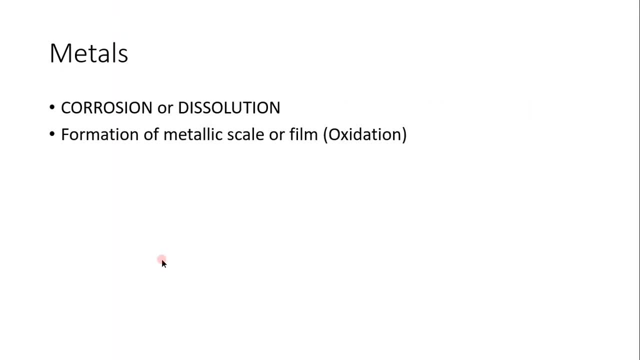 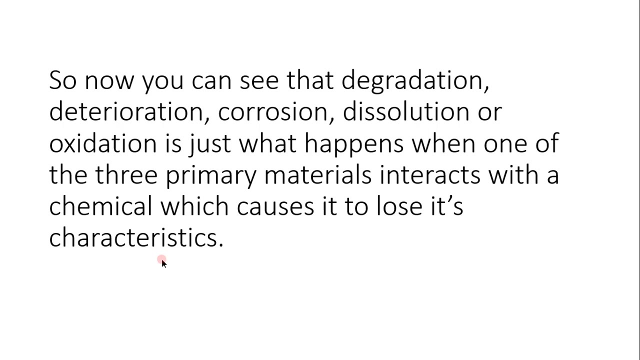 lose in dissolve. so that's how you can remember that metals dissolve. So metals either undergo corrosion or dissolution, as well as oxidation, which is just the formation of a metallic scale or film. So now you can see that degradation, deterioration, corrosion, dissolution or oxidation is just 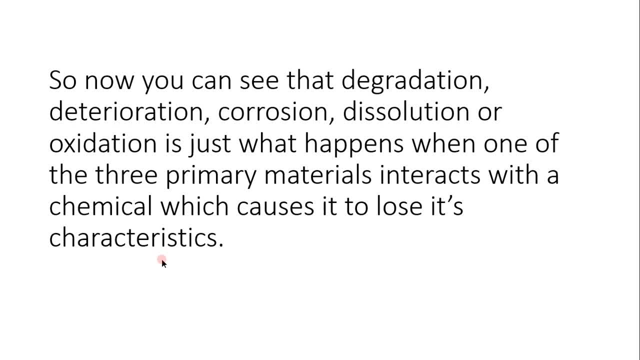 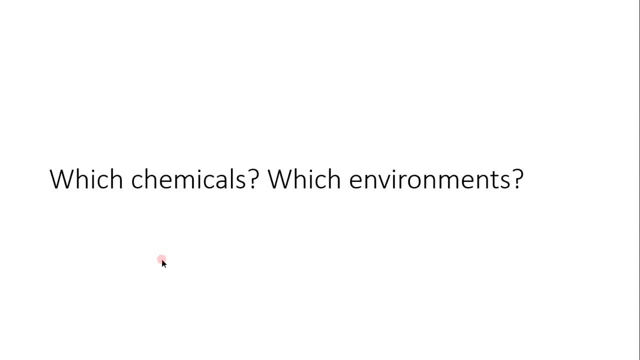 what happens when one of the three primary materials interact with a chemical which causes it to lose its characteristics? That's all it is, and they have special names to distinguish them. So you're probably thinking: okay, which chemicals, which environments? 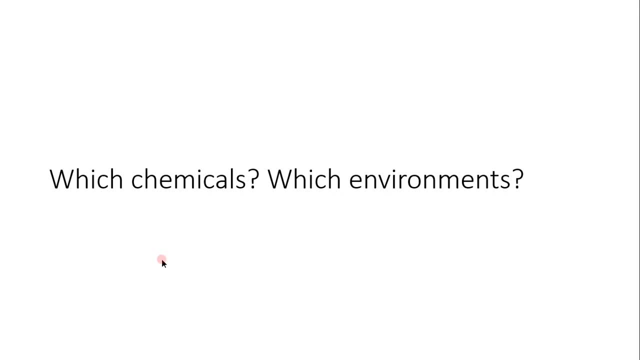 what do I need to watch out for with polymers, Like I understand, I sort of need to wear sunscreen, and you know, at the beach, so you know my DNA doesn't get destroyed. but what else you know? when, as an engineer, should I look out for when I want to build? 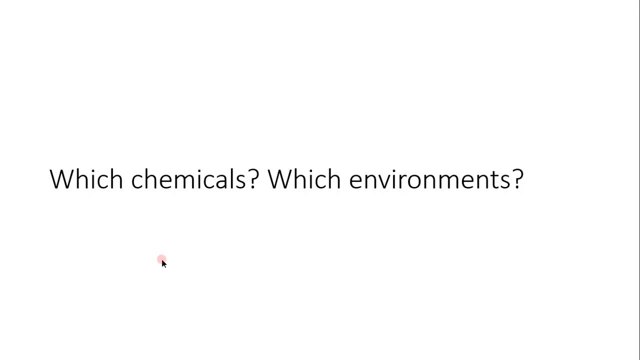 you know some kind of chemical? Well, that's a good question. So you know, as an engineer, should I look out for when I want to build? you know some kind of chemical? Well, as an engineer, I build certain things Which chemicals Like. if I want to build something in the